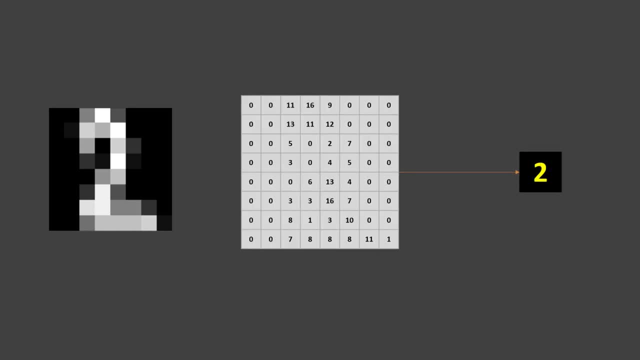 here this image is represented as pixel. let's say this is a grid of 8 by 8 and every number presents the color. so 0 means black, 16 means highest white, you know, and since it's an 8 by 8 grid, there are total 64 pixels, or numbers. that helps you determine what number it is. so these: 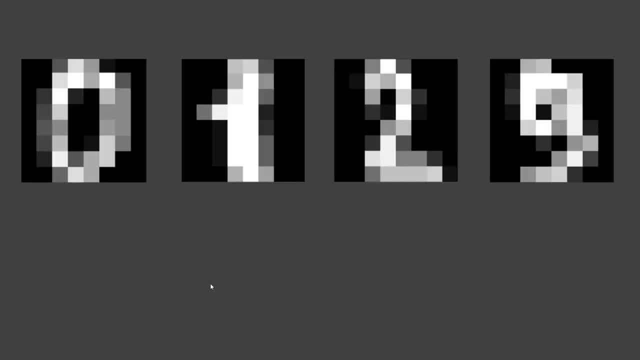 64 pixels are called features and if you represent now, if you think about some of the pixels in these images, you will find that those pixels don't play any role at all in figuring. what is it? what digit is it? for example, these two pixels here, or pretty much any pixel. 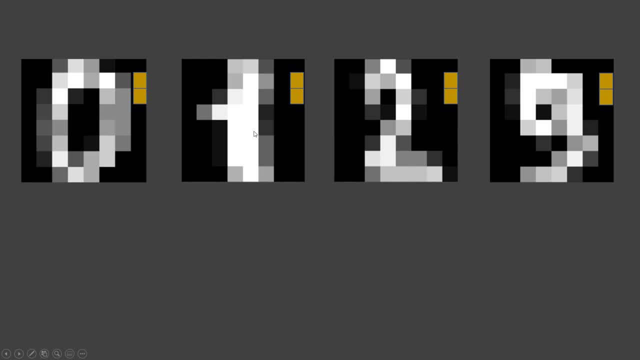 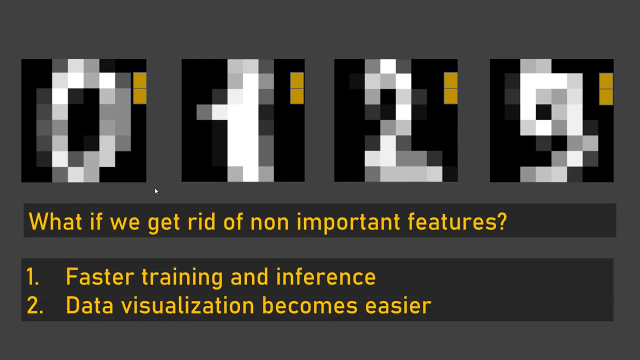 in this last column. no matter what number it is, these pixels are always black. so we can say that these pixels are not important feature. and what if we get rid of these features? we get two benefits out of that. first, the training is faster. you know machine learning. 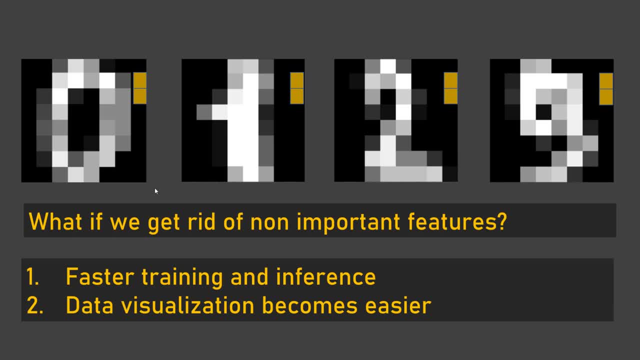 training takes a lot of time, a lot of compute resources, so you want to save the training, you want to make it a little lightweight and your inference can also be faster and data visualization becomes easier. let's say you have 100 features and somehow you want to. 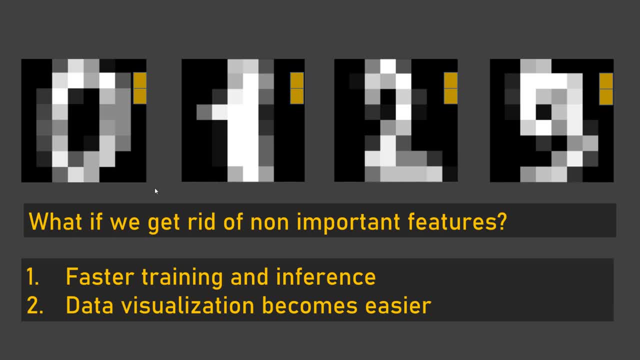 visualize how you reduce those 100 features into only two features or three features. then, as a human, you can plot it on a 2d or 3d graph, you can visualize it and data visualization helps a great. data visualization helps you a lot in terms of your final decision making. 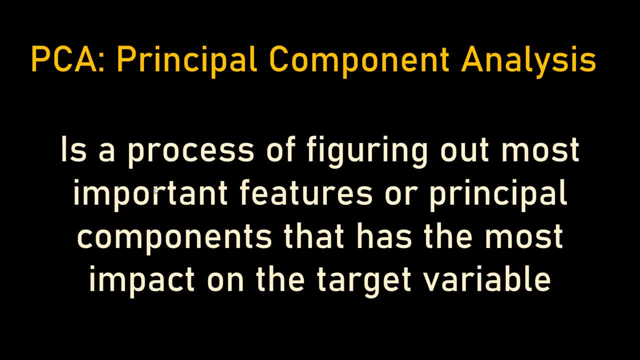 with regards to what kind of model you want to build. PCA is a process of figuring out the most important. PCA is a process of figuring out the most important. PCA is a process of figuring out the most important features or the principal component that has a maximum impact on a target. 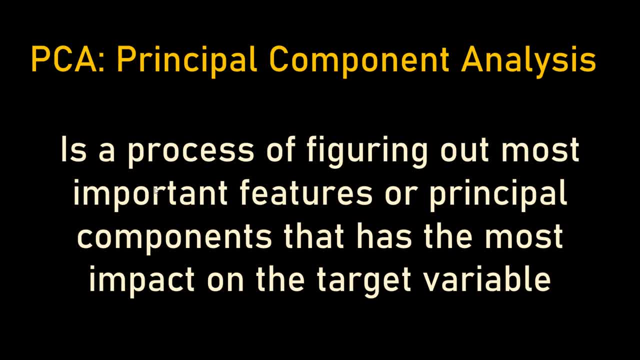 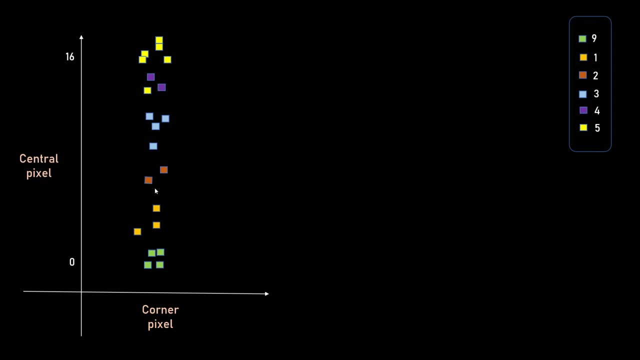 variable PCA will create, in fact, the new feature called principal component. you know PC 1, PC 2 and so on. so again going back to the digits example, let's say I have 64 features. out of that I am plotting only two features: corner pixel and a central pixel. now here, these cluster represent different digits. you 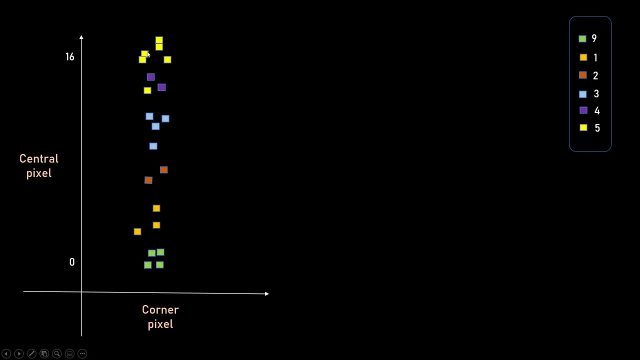 immediately notice that the corner pixel is not playing an important role. maximum variation is on the y-axis, or maximum variance is on the y-axis, which is a central pixel. so if I ask you to reduce this two dimension into one dimension, you can easily do so by getting rid of corner pixel. so this 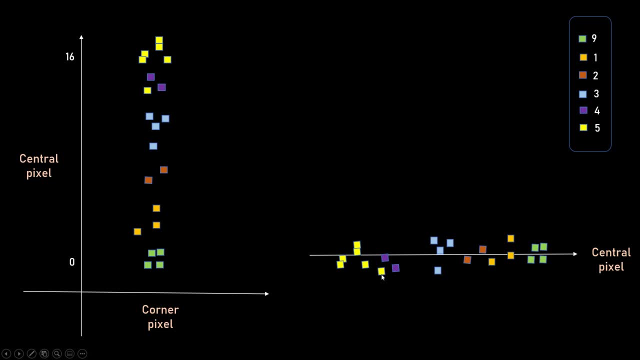 graph that I have drawn on the right hand side. it is one dimension. I mean, I know the graph is not perfect, it still looks like two dimension, but you get my point. to reduce this from two dimension to one dimension is easier. let's look at the iris flower data set. 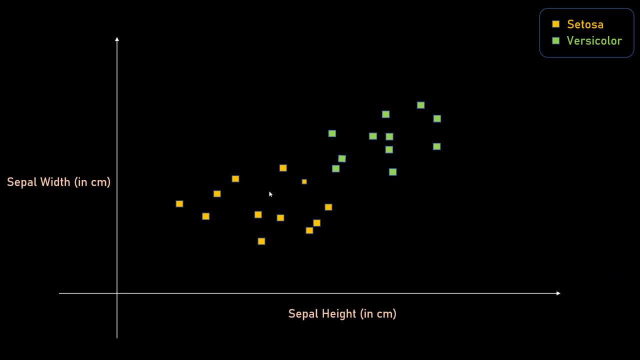 where sepal width and sepal height determine what kind of flower it is. if you have a scatter plot like this, you can draw a line which covers the maximum variance. so this line covers the maximum variance, or the maximum information in terms of features, and you can draw a perpendicular line which covers the second most variance you know. 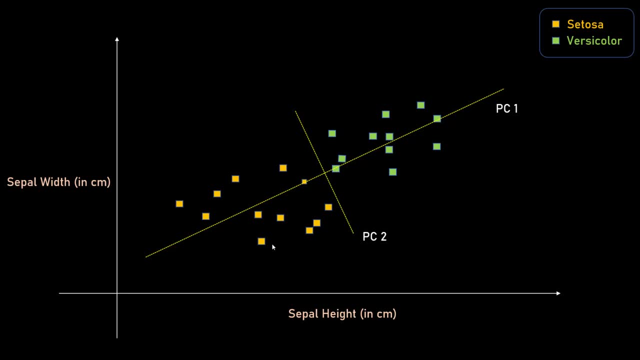 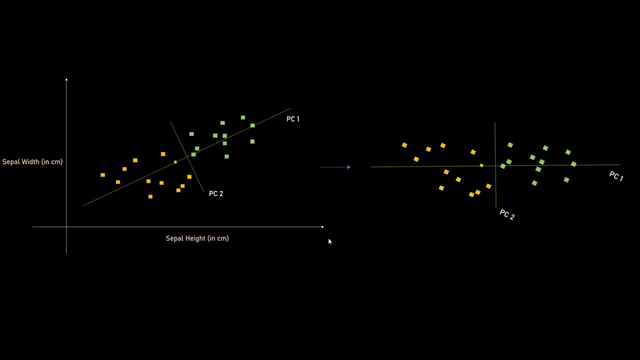 and these are called principal component. so here, PC1 is this axis which covers the most of the variance. PC2 is the axis that covers the second most variance. so when you apply PCA you get a chart like this and I know I have done only in this. 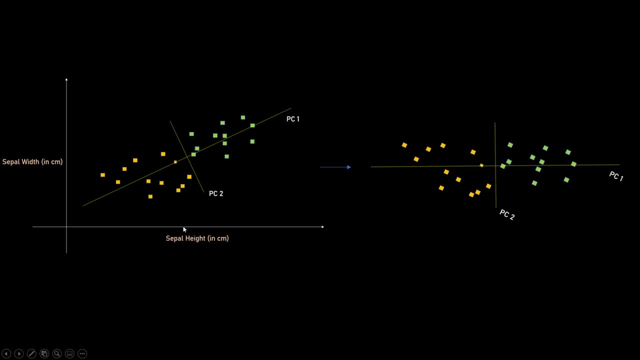 graph for two dimension. but really if you have hundred dimension and if you apply PCA you can figure out, let's say, ten most important piece principal components. so for hundred features you can actually create hundred principal components in the descending order of their impact on the target variable. 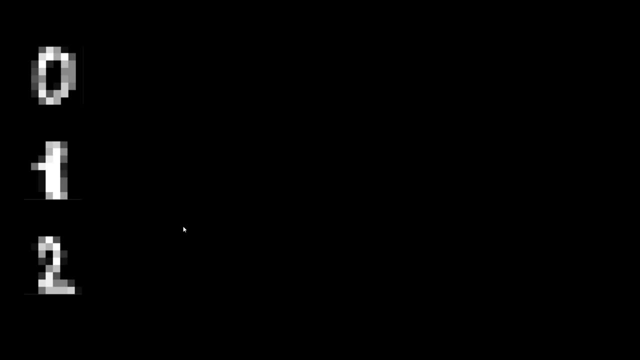 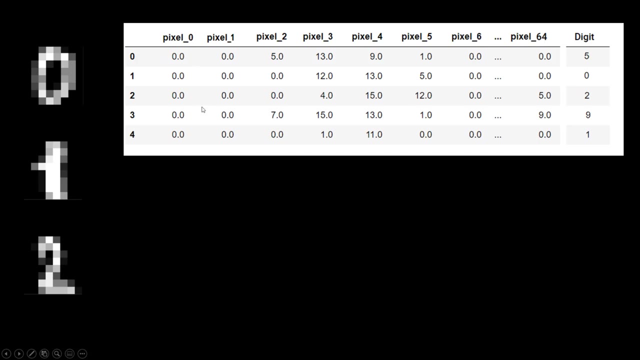 you can see that this is the number of values, very important number of values on the data frame and in fact, this is the number of values of the data frame. so for digits, if I have to load this in a data frame, Pandas data frame will look. 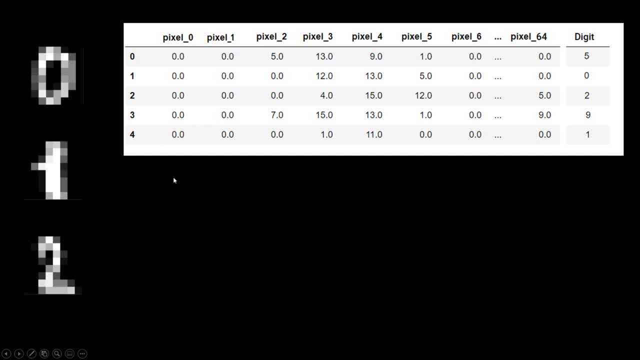 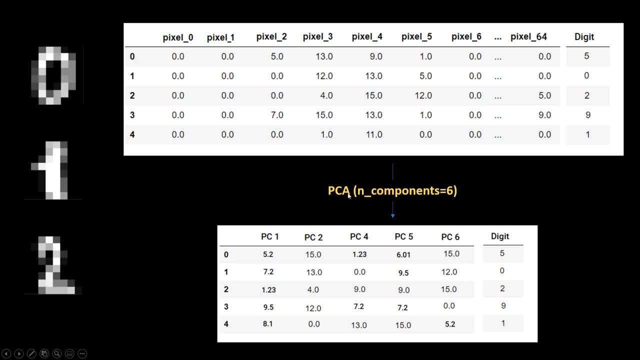 like this. there's a little error, is like pixels 63, because I start with pixel 0, but you already see pixel zero and one has all values is zero. they are not kind of important. so when you use a scale on library and call PCA method, where you say: 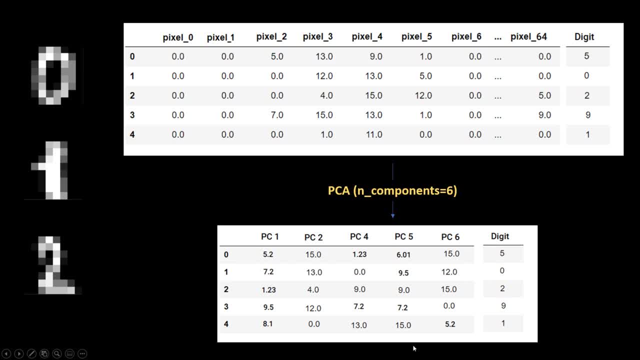 okay, and components is 6, you're basically asking PCA to extract the 6th, most important and fixed values component, and that will look something like this: so what this is doing is calculating new features and these features are such that PC1 covers the most variance in terms of features. you know, in terms of information extraction. 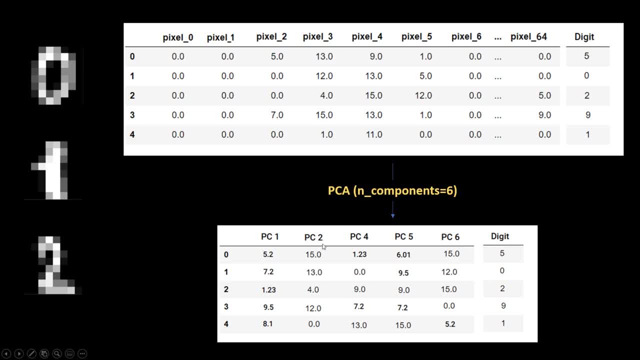 from your data set. PC2 is the second most highest component that contains a lot of information about the features of a data set. here I give six. you can give it anything. you can have two, three, four, five. you know trial and error. you can also give a different parameter to this method, which will be like 0.95, which. 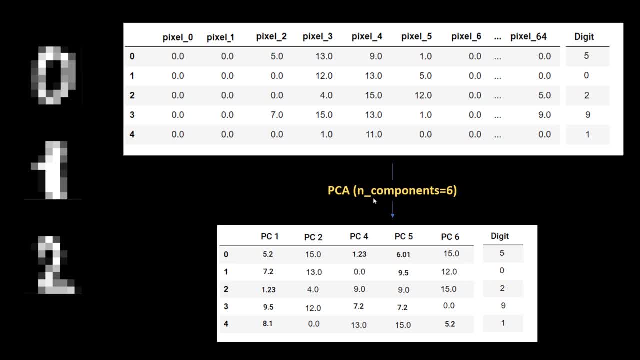 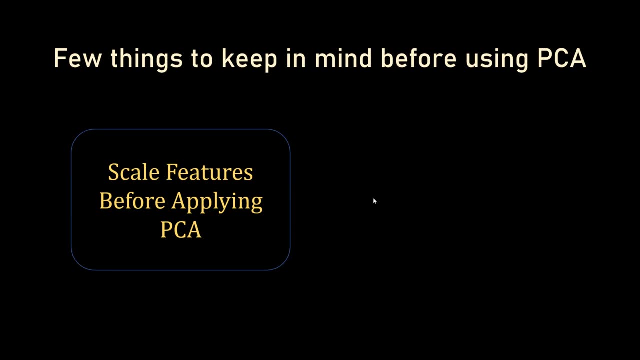 which means, you know, get me 95% of information in terms of features. you know, get me 95% of variance. so you can do that. we'll see that in the actual coding section. but few things to keep in mind before using PCA. is you need to? 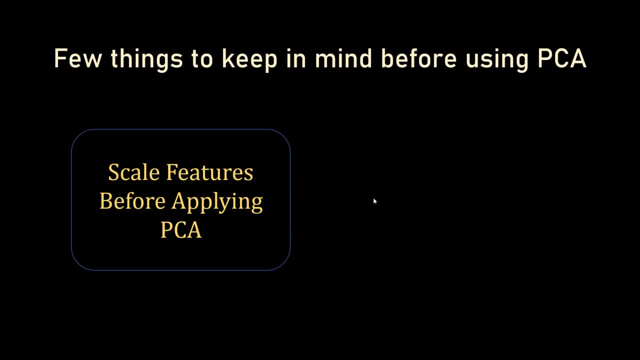 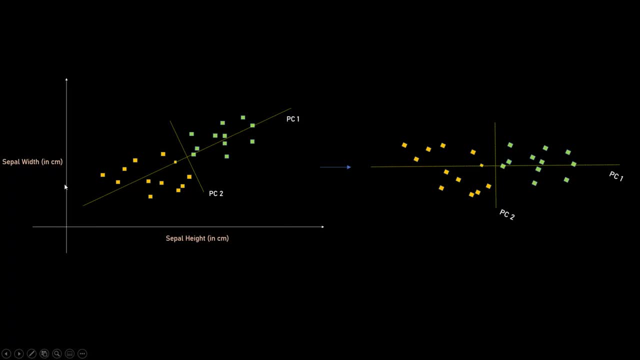 scale the feature, because if you don't scale it it's not gonna work. okay, for example, here is a chart and if this graph is in millions and this graph is in a normal value, you know the graph might become skewed and PC and the PCA will not work as per your. 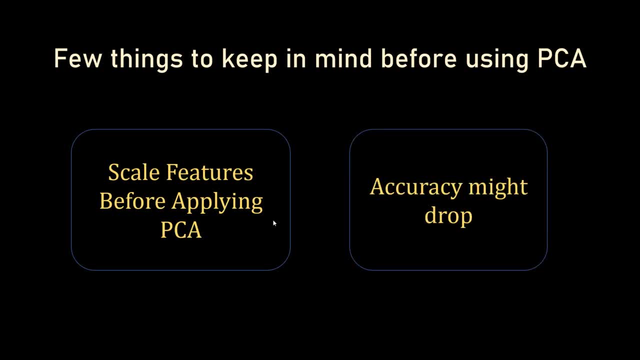 expectation accuracy might drop. so it's a trade-off. when you're trying to reduce, let's say you have hundred features and if all hundred features are important and they're trying to reduce the number of features that you're trying to reduce to contribute to and target variable, if you reduce from hundred to five you're. 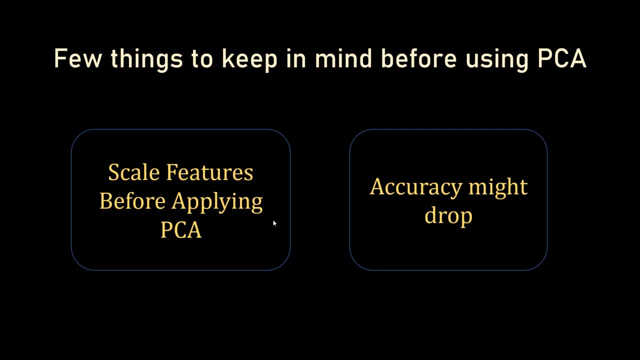 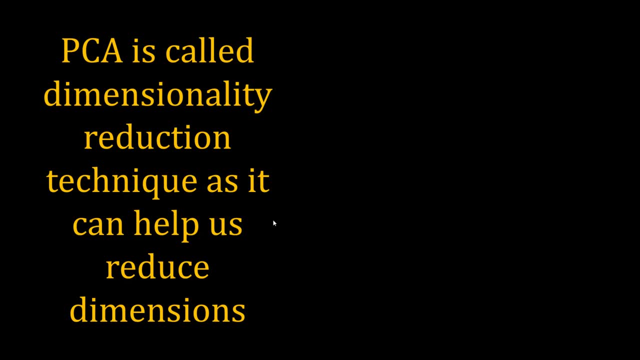 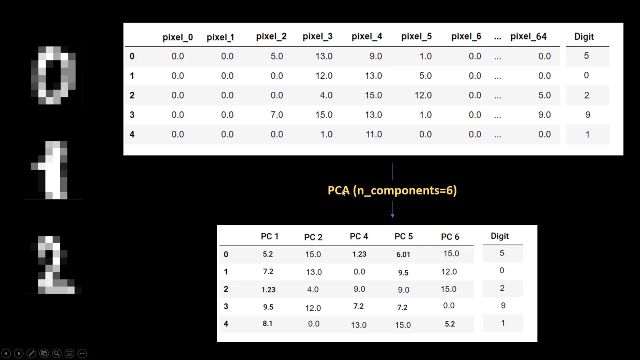 going to lose a lot of information. so we'll see all of that in the coding session. but just to summarize, PC is called a dimensionality reduction technique as it helps us reduce dimension. we already saw here. in this case we had 64 dimension. this helped us to get to six dimension, and when you have 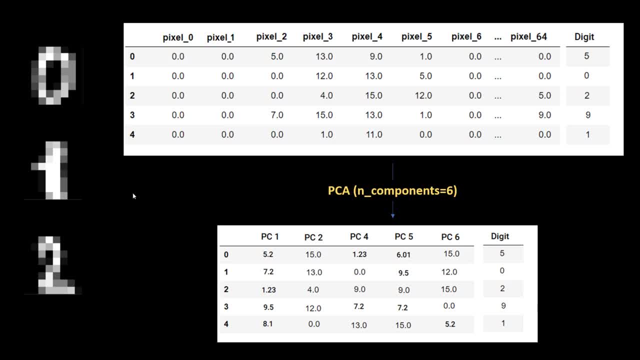 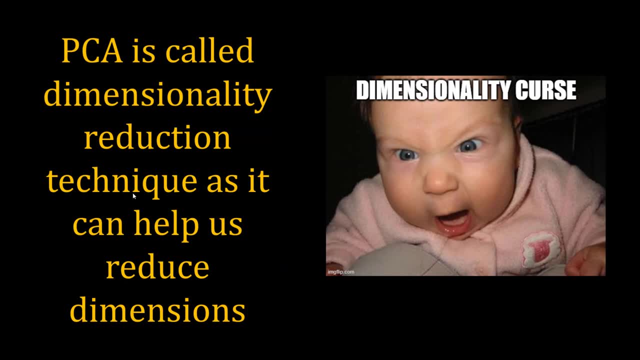 less columns, your computation is going to be much more efficient, becomes much faster And it also helps you to address the dimensionality curse problem In machine learning. dimensionality curse is a big problem. So many datasets having so many, so many columns. you know so many. 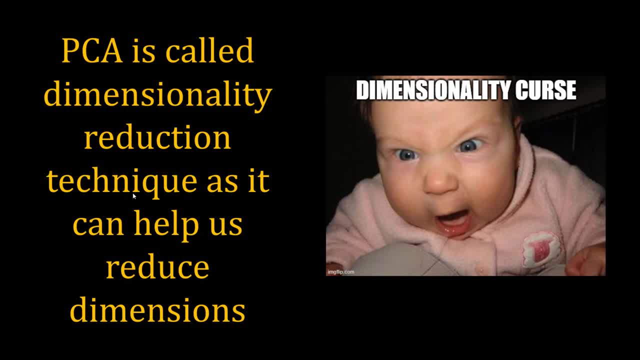 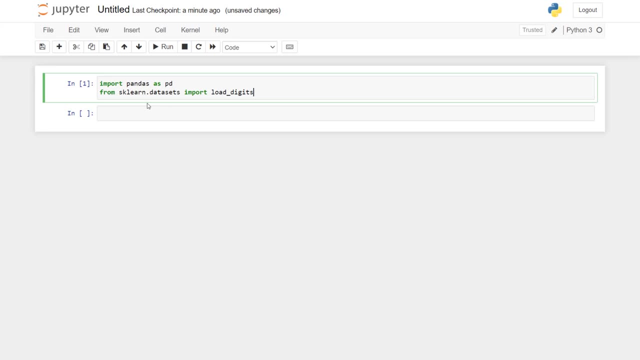 dimensions and that makes our model really complex, hard to visualize, and PCA is an excellent technique that help you deal with dimensionality curse. Let's get to Python coding now. I opened my Jupyter notebook and imported some important libraries. I'm going to use the handwritten digits, data set from: 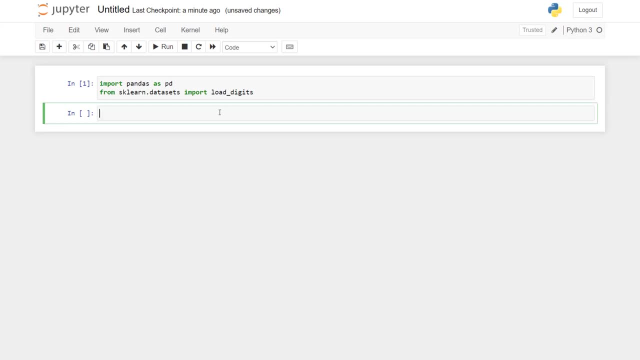 sklearn data set module. Let's load the data set by calling loadDigits function. When you do that, it loads the data set and you can call data set dot keys to get an idea on. you know what the data set is all about. You can see that. 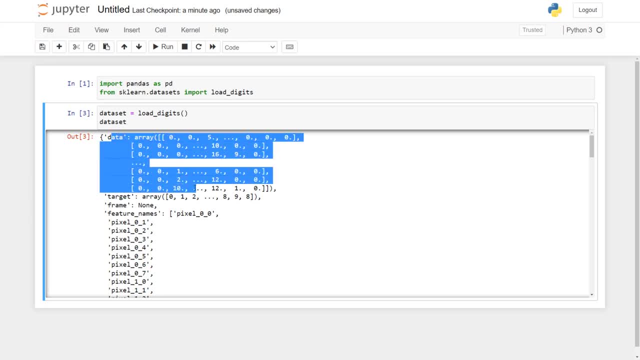 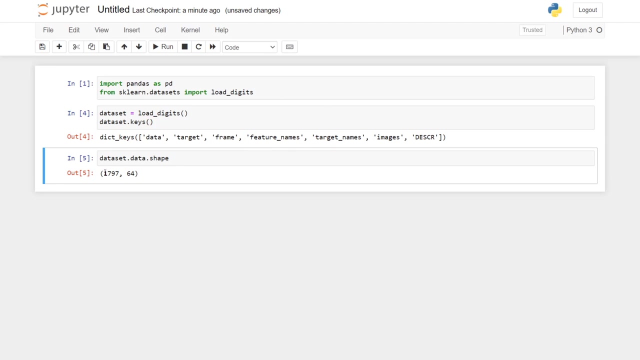 data set dot data will contain all the pixels and these are the feature names and this is the target array. right Now let's look at data set dot data dot shape. So there are 17, almost 1700 or 1800 samples. Every sample has 64 columns, So 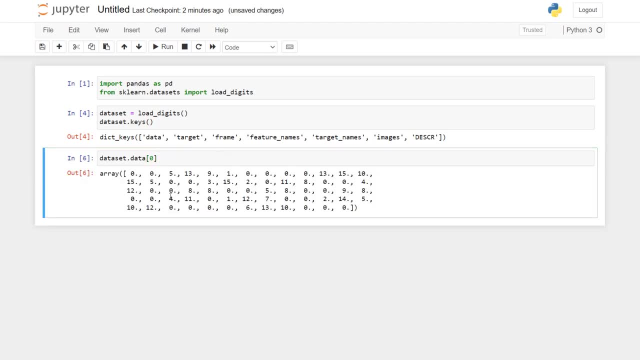 if you look at the first sample, it's a flat one-dimensional array of 64 pixels, and if you want to visualize this data using matplotlib library, you need to convert it into two-dimensional array, and the way you do that is by calling reshape function, because this is numpy. 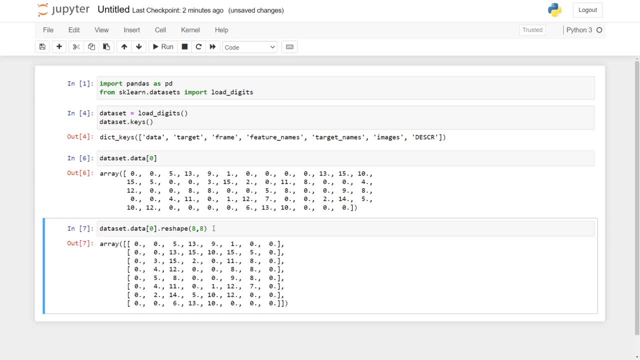 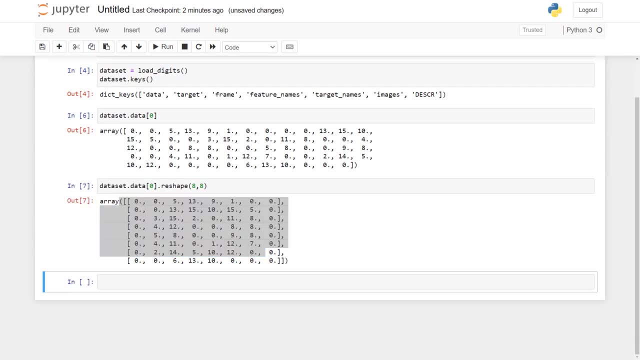 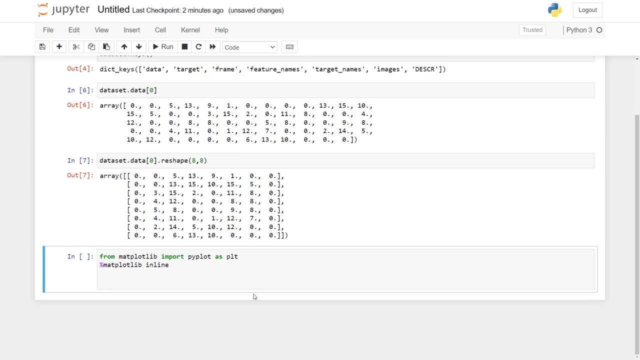 array and when you do 8 by 8 it just converts one-dimensional array into two-dimensional array of pixels. Now you can import matplotlib and use the plot. You know, I'm gonna just plot a grey image And when you do plot dot mat show like metric show, it will show that it will show a picture of that. 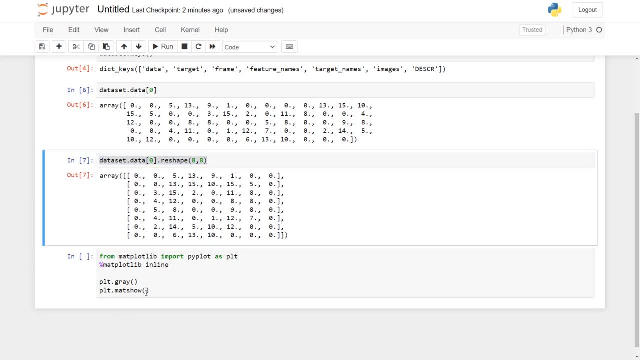 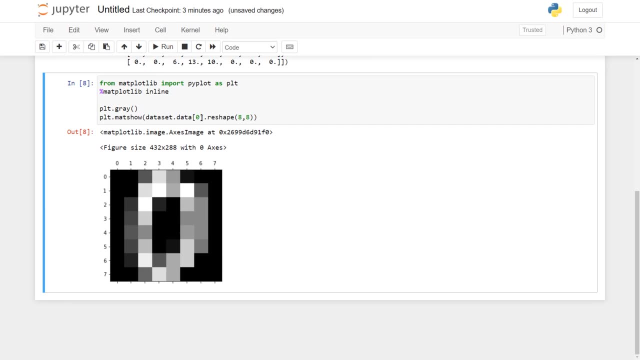 array. what is my array? this is my array, right, see two-dimensional array. so I'm gonna just put ctrl-c, ctrl-v, and my first digit looks like this: this is clearly 0.. If I load the data set by calling reshape function, it shows exactly this same thing, like 0.. 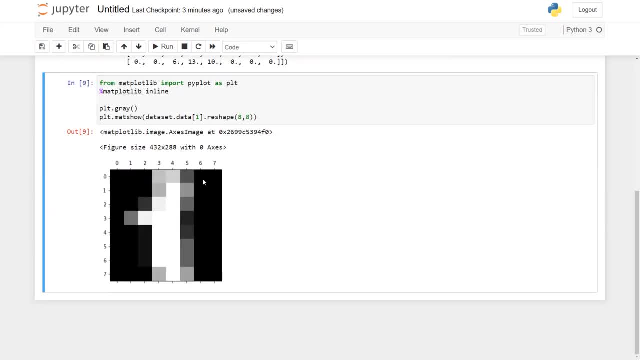 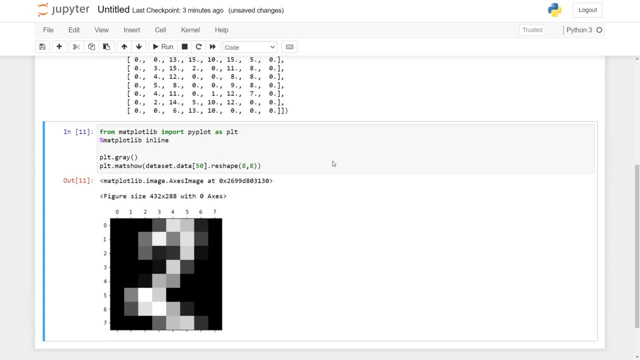 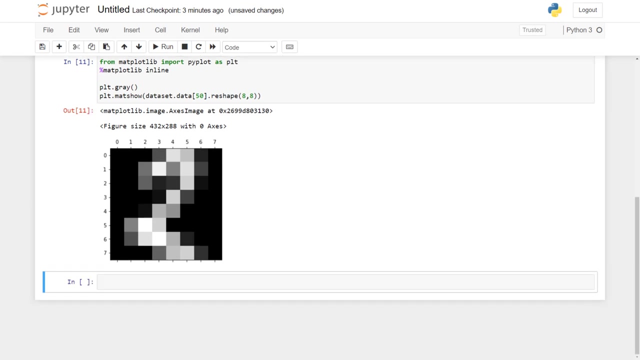 look at my second data sample: see it is 1, then 2 and so on. you know like 50th sample will be. I think this is 2. okay, so this is how you visualize it. now let's look at the target. when you do data set, dot target. it's a huge array but it is. 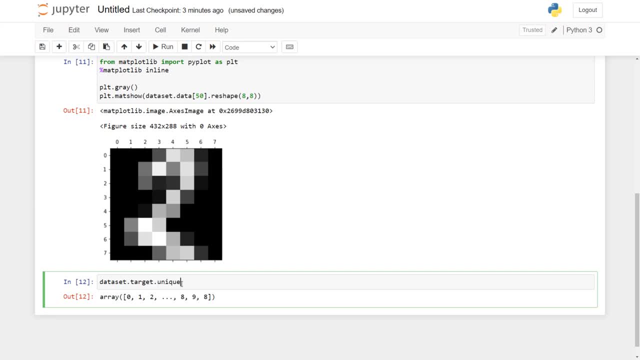 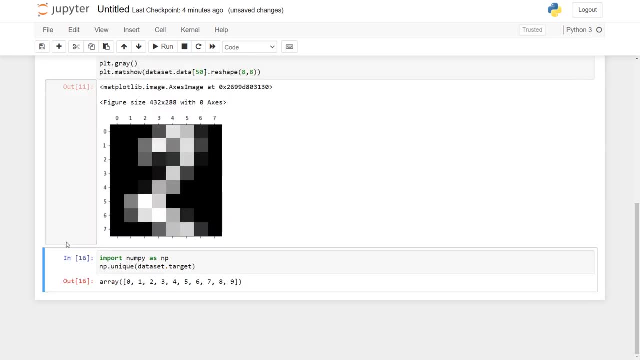 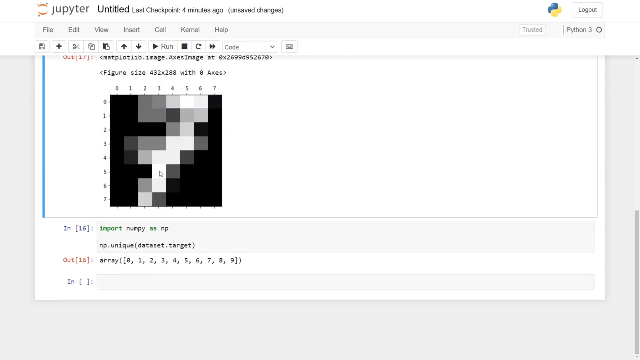 your end class. you know if you do unique you will find. the way you do unique is by calling NP dot unique and you see the numbers are between dreams 0 to 9. we already saw, let's say, our 8 number. here is which number it is. okay, I can check it here. 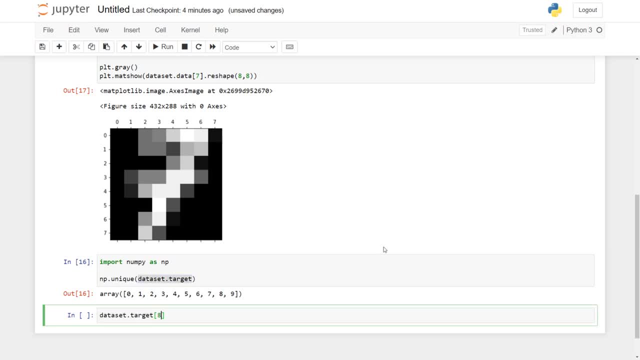 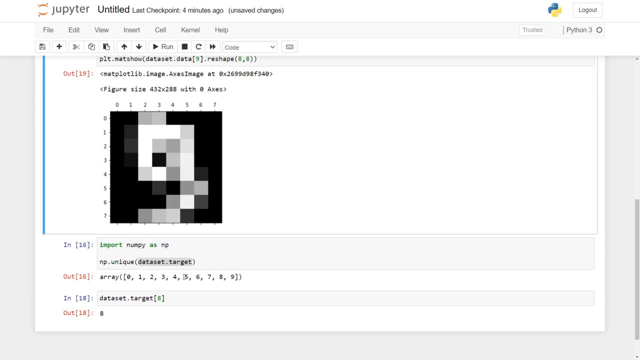 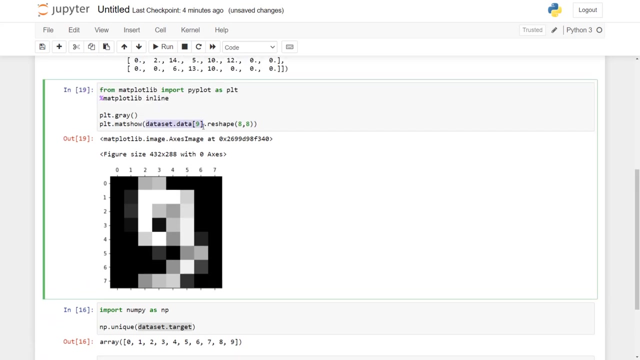 so if you do 8, this is the 8 number. I mean, I know it looks weird, but let's do the 10th number. so 10 number is 9: see 9. so this data set dot data is your feature and data set dot target is your class. basically, we are classifying this. 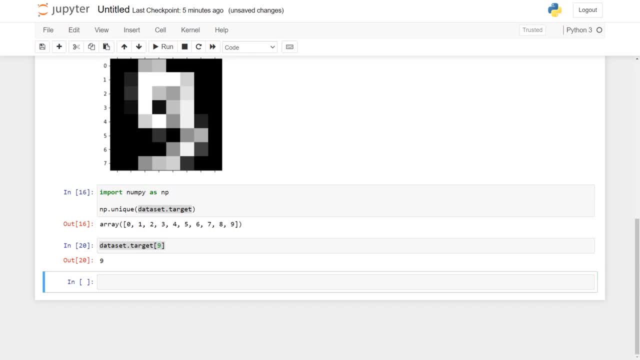 in 10 classes 0 to 9. okay, let me classifying this in 10 classes 0 to 9. okay, let me classifying this in 10 classes 0 to 9. okay, let me create a data frame now so I can do PD dot data frame and just supply data set. 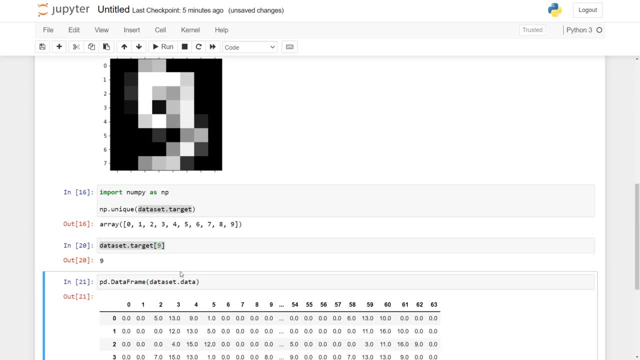 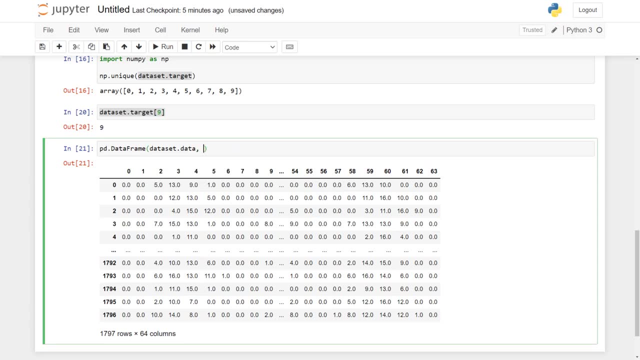 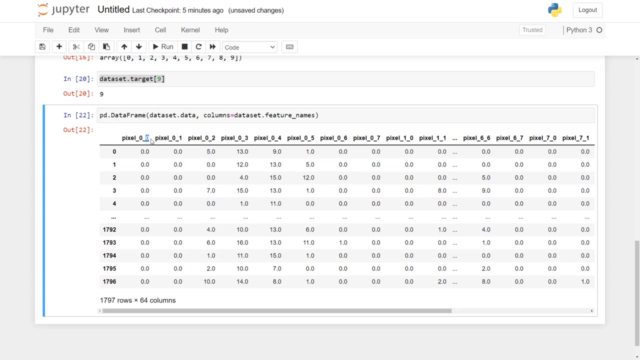 of data here and that will create a data frame for you. but the column headers are, you know, randomly assigned. so I'm going to do columns. you can say data set dot, feature names. the feature names are all the pixels, you know, like: 0 throw 0 pixel. 0 throw first. 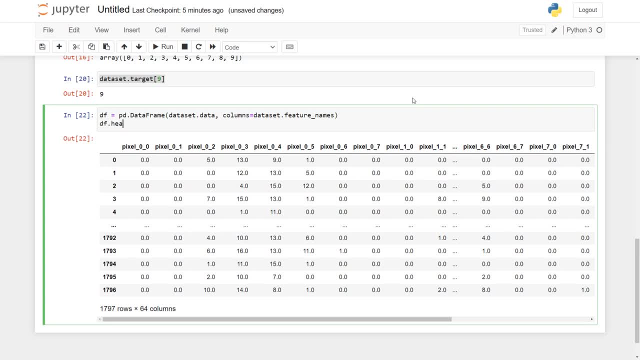 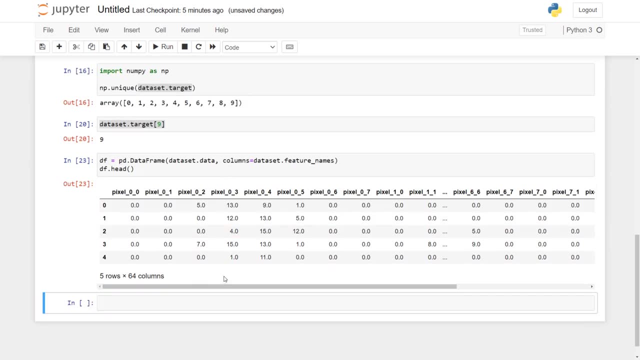 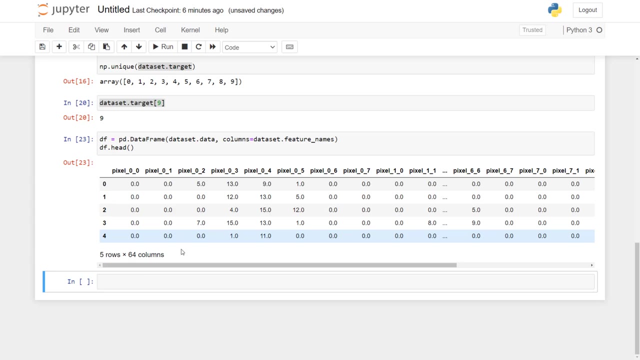 pixel and so on, and I will just save that into a data frame object. okay, my data frame object is ready now. I mean, I know from this data set the values are between 0 to 16, but if you want to confirm you can do df, dot, describe and. 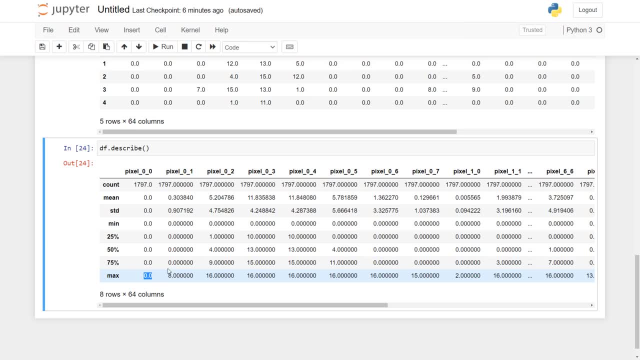 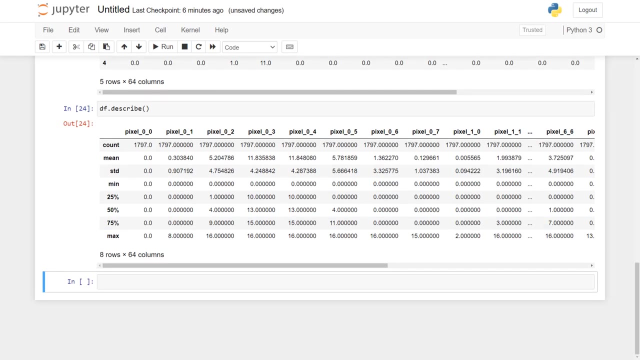 for each of the columns. if you look at min and max, I mean, this column is useless. but if you look at min and max, for most of the good pixels it will be between 0 and 16. okay, so 0 is my minimum value, 16 is my highest value. now I am. 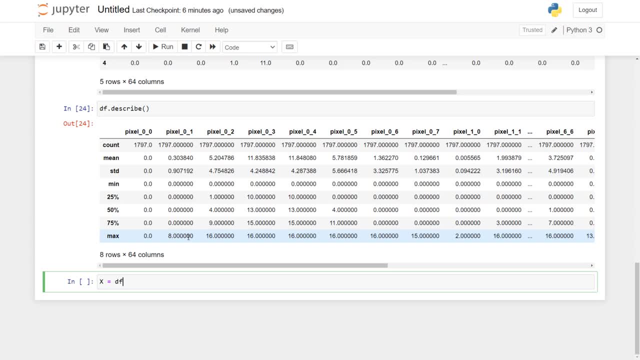 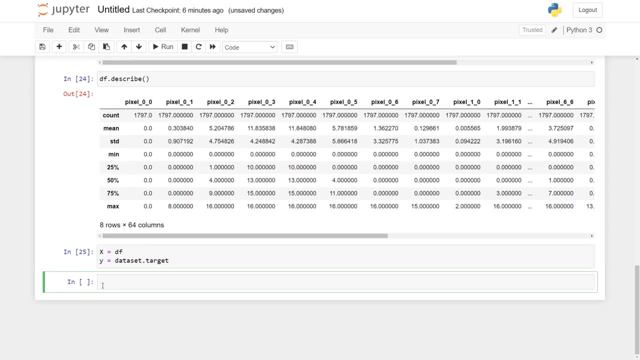 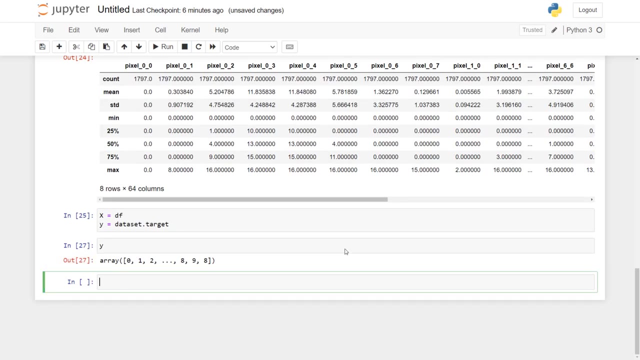 going to store this in X and y. so DF is my X and my Y is my unit target set. so again, what is my X? X is my data frame. what is my Y is my target classes. you know the digit which tells you zero, nine. now I would like to scale these. 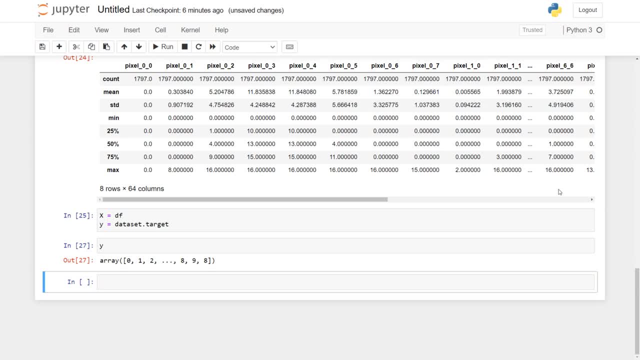 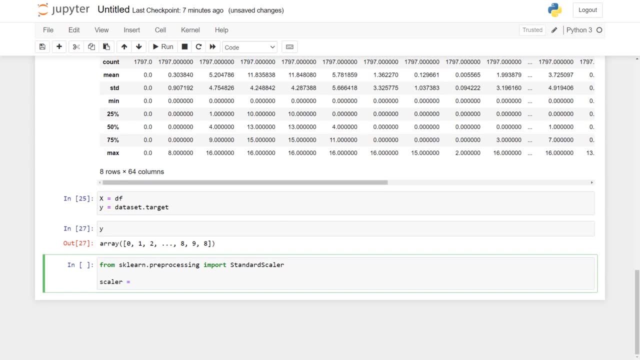 features before building my machine learning model. so I'm just going to use the standard scaler. you know scaling is a common thing that I do before training my model model and a scale and provides very convenient API to do that. when you do scalar dot fit transform, it will just scale that X thing and you can store. 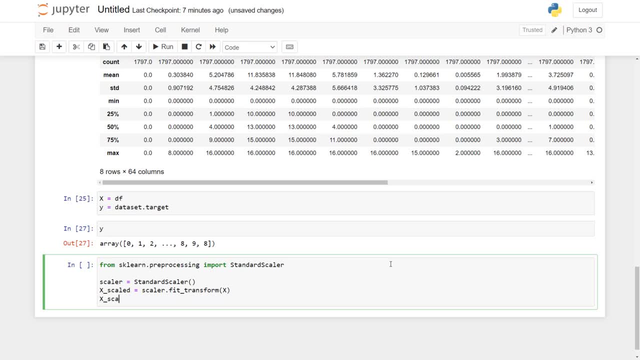 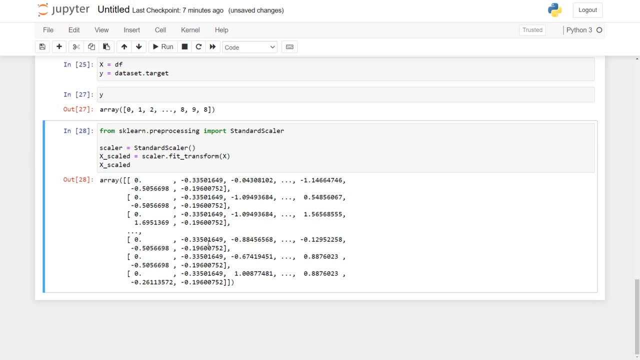 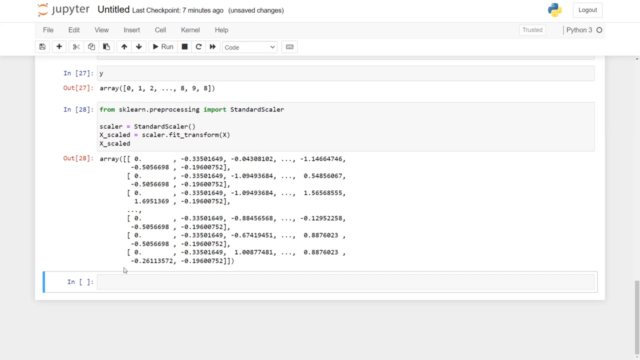 this into X scale. so when you print now X scale, you will see the values are stand their scale. you know, using the standard scalar- I think negative one to one- you can use min max scalar as well. okay, now we are ready to train the model, so we are going to do a usual thing, which is train this plate. you 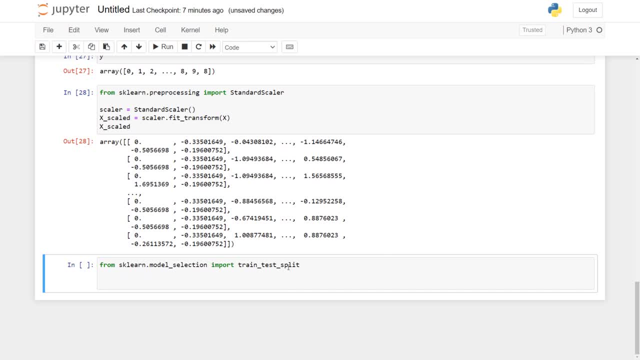 already know this. but by this, not by this point, and I'm going to call train this plate on my X scale. so X scale and Y, and I will keep my taste size to be 20%. you can do 30%, whatever, and I'm just keeping random state for reproducibility. 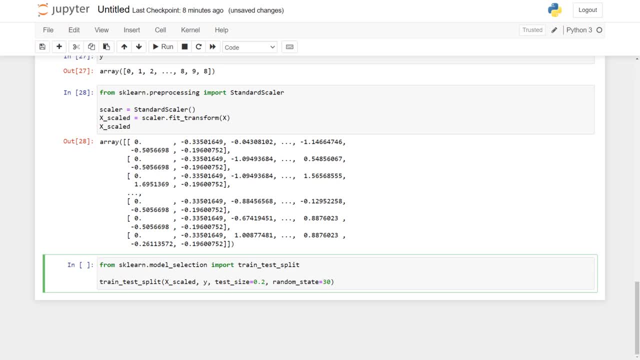 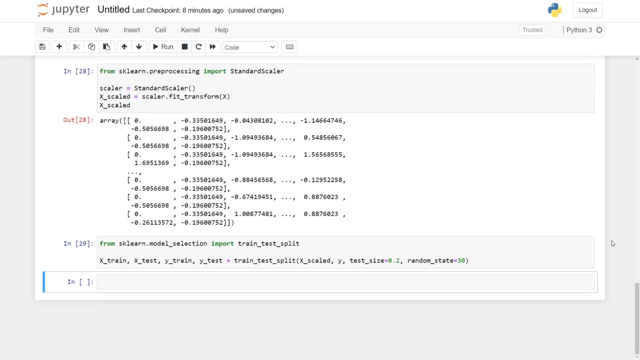 if you don't want to keep, it is fine. and in the result, what I get is X train, X taste, Y train, Y taste. this should be in your muscle memory, friends, if you're doing machine learning for some time. now I am ready to train my model. well, I am. 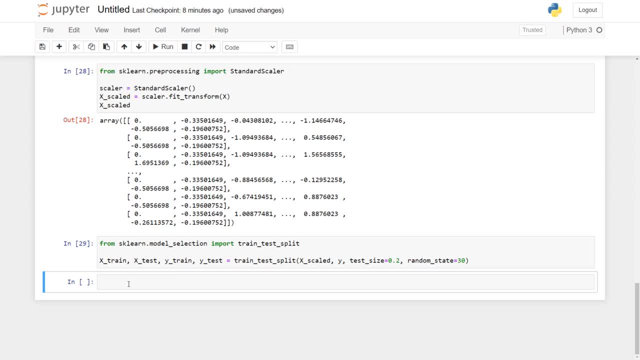 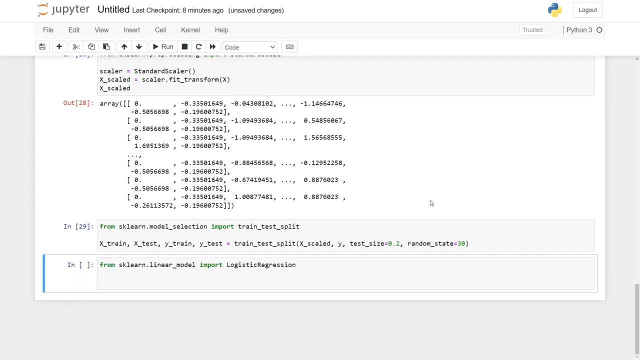 going to use logistic regression. you can use a random, for, as this is entry, there are so many classification techniques, but I'll start with logistic regression. I will create a model which is an object of this class and then model dot- fit again pretty standard- and model or score. so I do model or score to measure the accuracy. 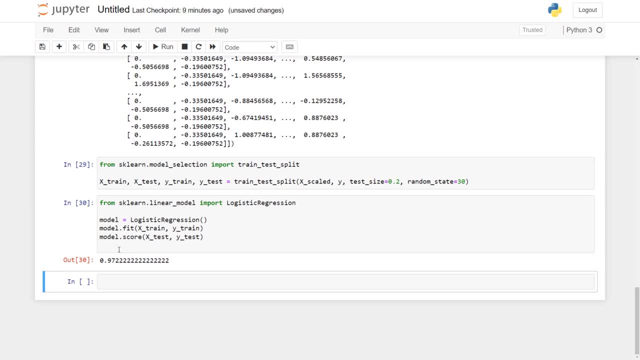 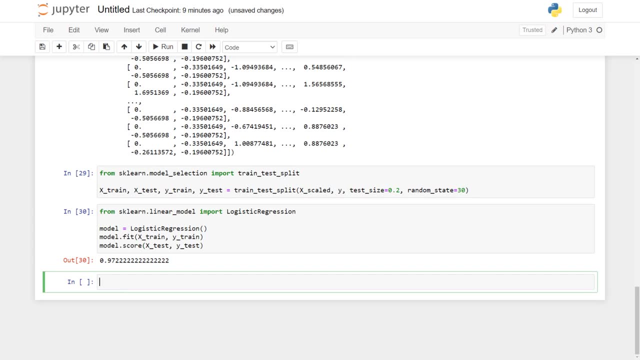 you 97%. see, this is pretty amazing. I get 97% accuracy by training on all these features. but now let's do PCA. so to do PCA, you can import PCA from SK. learn decomposition and then I will create a PCA variable. so let me increase. 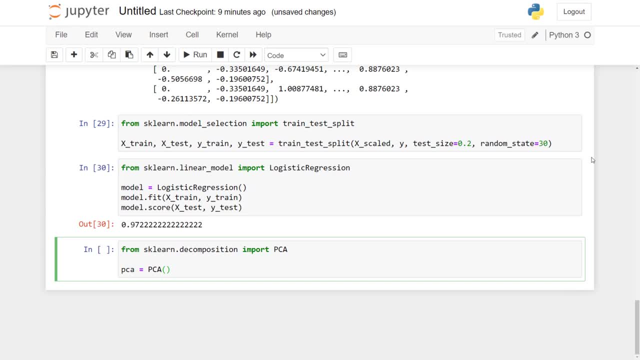 my font size. it's very simple: PCA. and here you supply two type of arguments. you can either say how many components you want, you can say two, five. trial and error, you can figure it out, but what I'm going to do is I'm going to supply 0.95. what this? 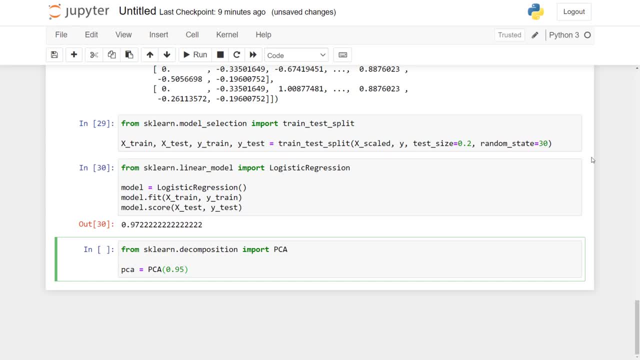 will tell PCA is that: retain 95% of useful features and then create new dimensions. you're not explicitly saying: I want only two dimensional as an output. you're saying: give me, retain 95% of information, retain 95% variation and then whatever features you come up with, I'm happy with. 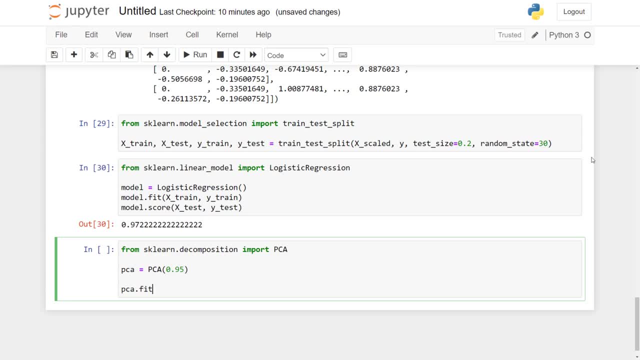 that and then PCA dot fit transform. the API is quite simple. you supply your data frame here, you get a new data frame with new feature, new principal components, and when you do X PCA dot shape- see now you got only 29 columns. I'm gonna define a new detail. 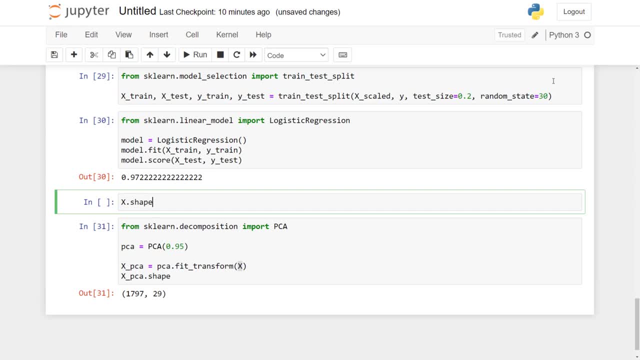 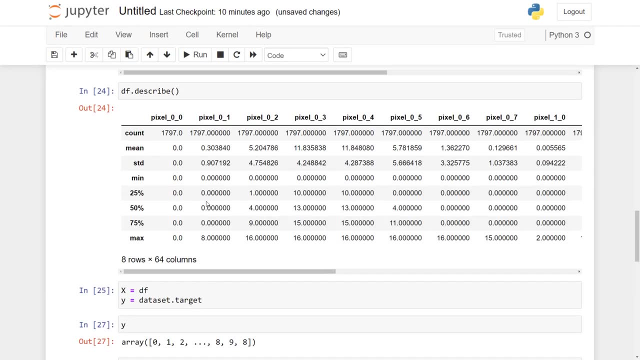 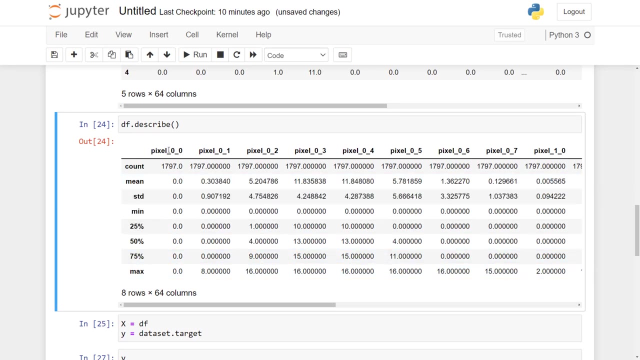 if you look at your original data frame, you had 64 columns, so 64 columns to 29. it probably got rid of unnecessary things such as this guy, for example: see 0 pixel. all values are 0. see, look at here. this feature is not needed at all. 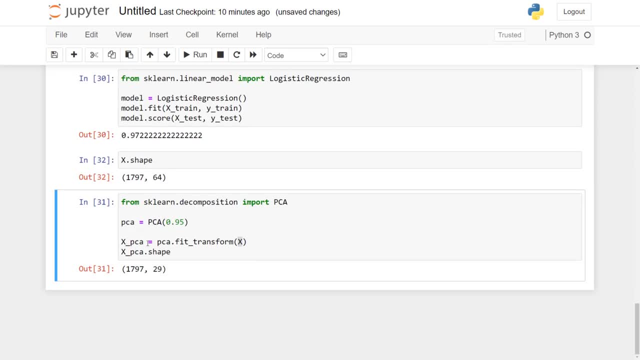 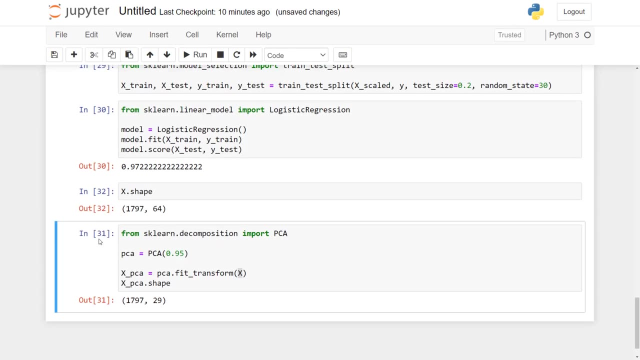 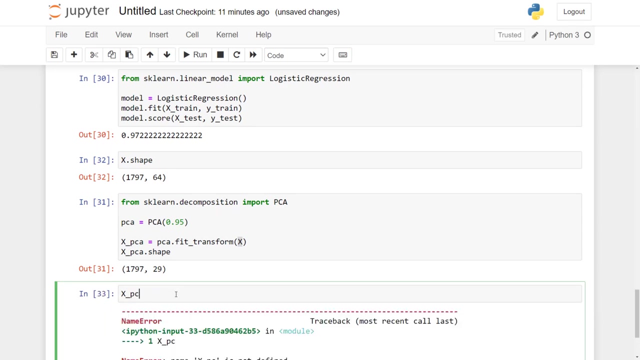 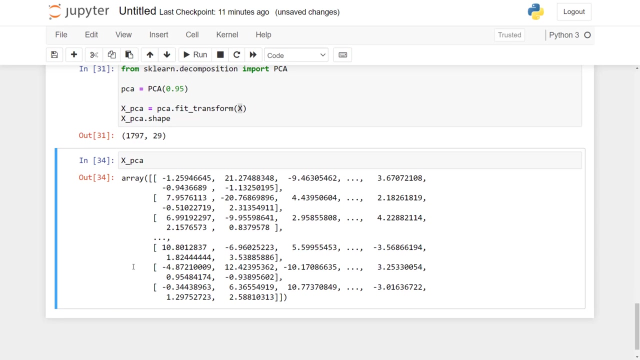 so it probably got rid of that and it it did not. by the way, just to make it clear, it's not like it will pick 29 columns out of it. it will calculate new columns. okay, so if you do X PCA, you see it actually calculated new columns for you and if you do PCA. 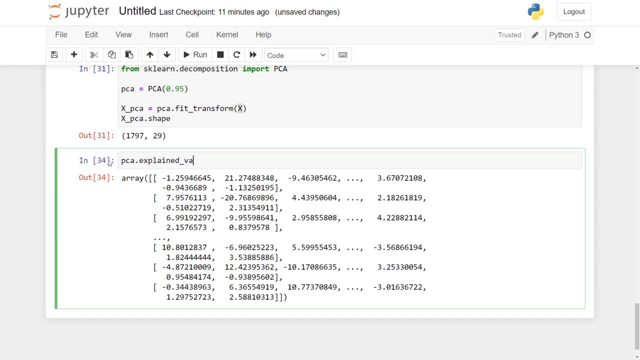 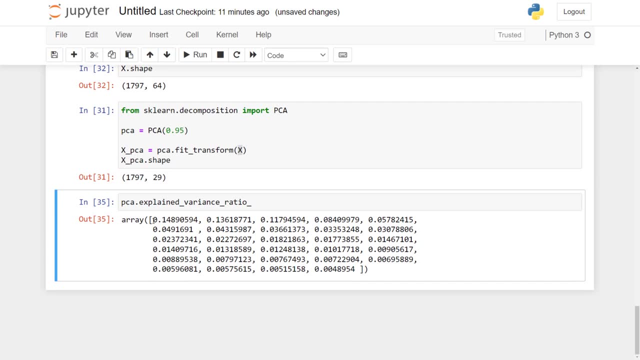 variable dot explained variance ratio. it will tell you that my first column is capturing, you know, 14 percent of variation, or 14 percent of useful information from my dataset Pc2. second component is capturing 13 percent of information and so on. so this is how you print explain variation ratio. there is another thing called n components. it 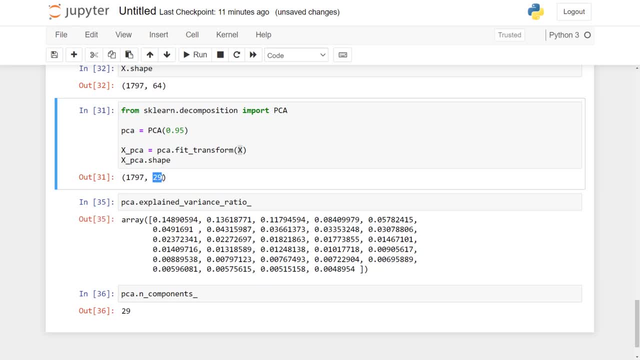 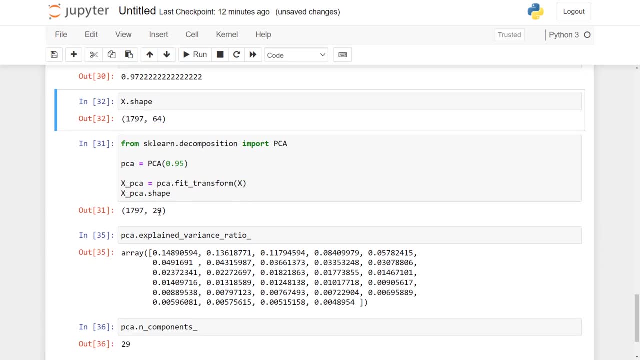 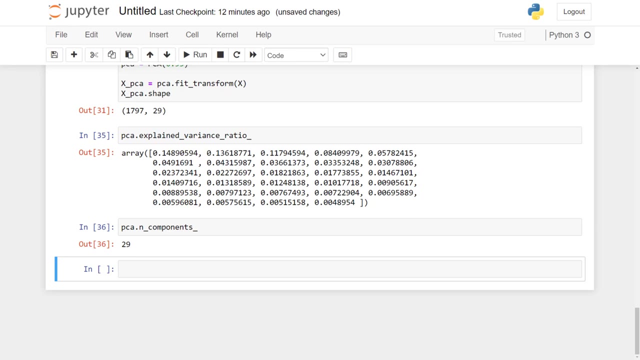 will tell you how many components you guard, which is basically your columns. you know 29. so here pca helped me reduce my columns from 64 to 29. all these 29 columns are computed column. they are the new feature. but good news is you can now use this uh new data frame to train your model. so i'm going to do train test split once. 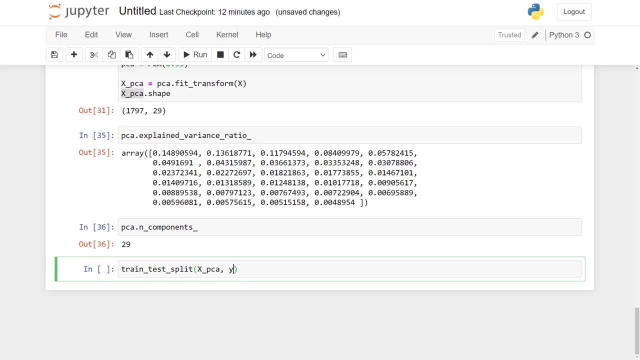 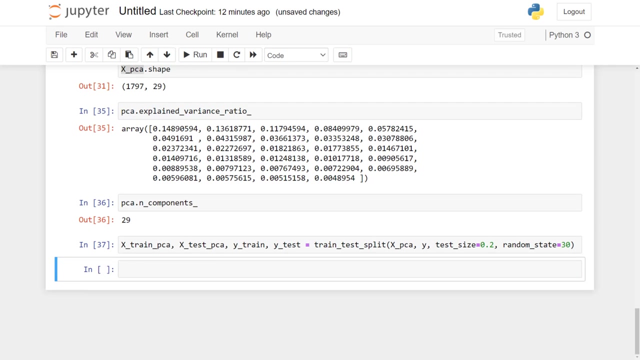 again, but this time i will supply x, pca, y remains y, then my test size is 0.2 and i'll just keep my random state to be this and, as a result, what you get is your train and test data sets and i'm going to use again same linear regression, logistic regression, sorry- and i will say: 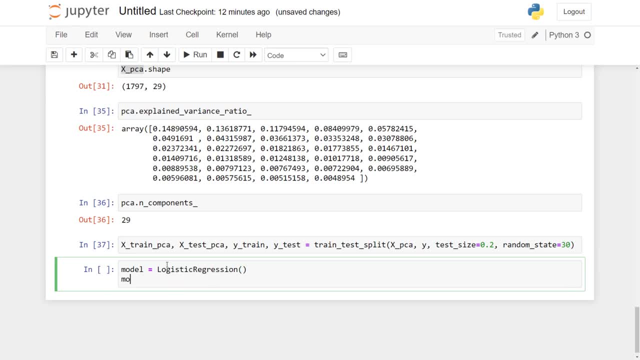 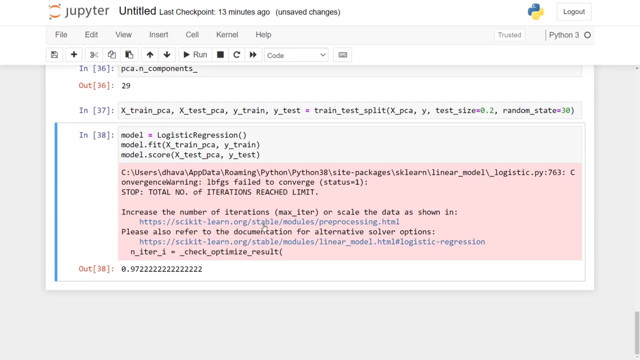 logistic regression. this time i will fit on pca and then model dot score and y is say i got pretty good accuracy, 97. but let's say this failed to converge because total number of iteration limit reached. so i need to supply some maximum iteration. so i will say 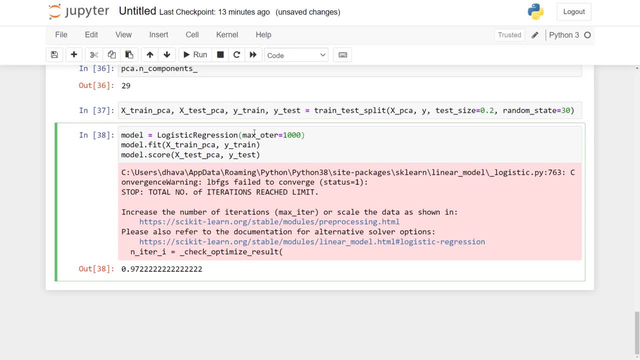 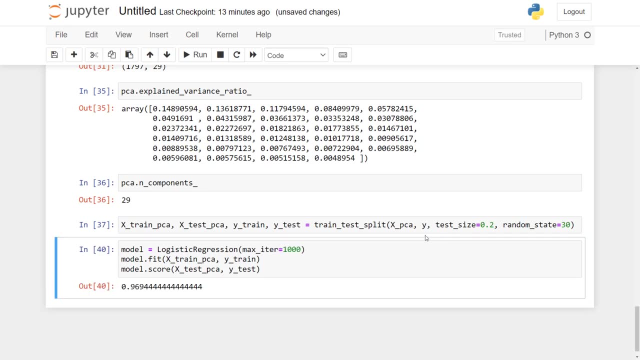 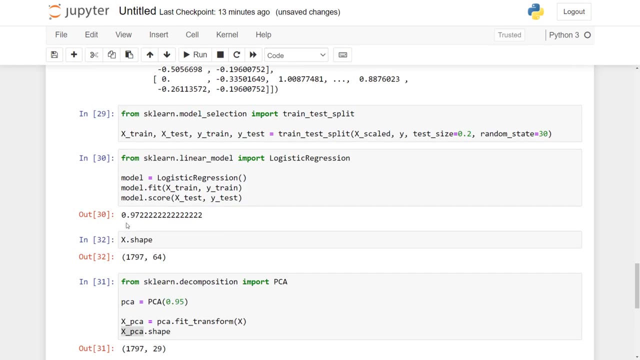 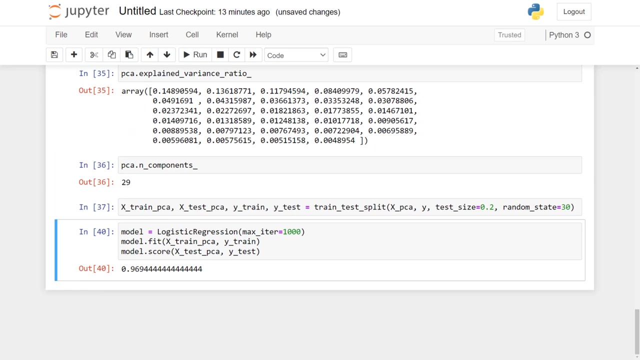 max iter. so i need to increase my iteration, basically to uh, so that the gradient descent can converge. see almost same accuracy. so you are realizing that, despite dropping a lot of features, my accuracy is almost same. here is 97.22, there is 96.994, so it's almost similar, okay. 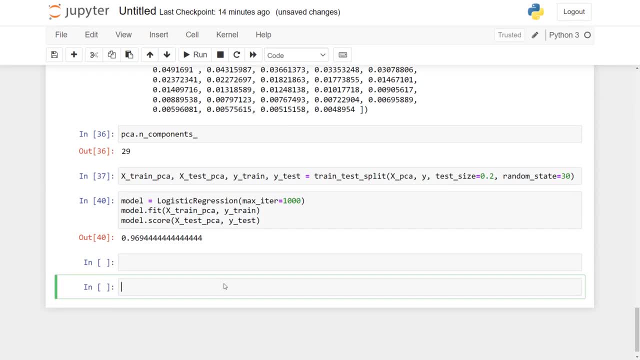 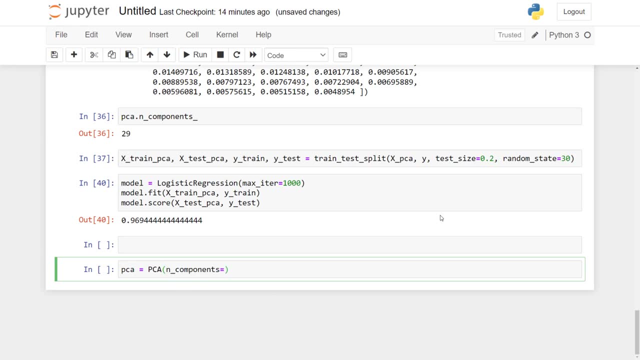 now you can um create pca by supplying the components explicitly so i can say: okay, pca. let's say my number of components is 2.. now this is what is going to happen when you explicitly say: my components are true, so i'm going to do pca transform with my x. 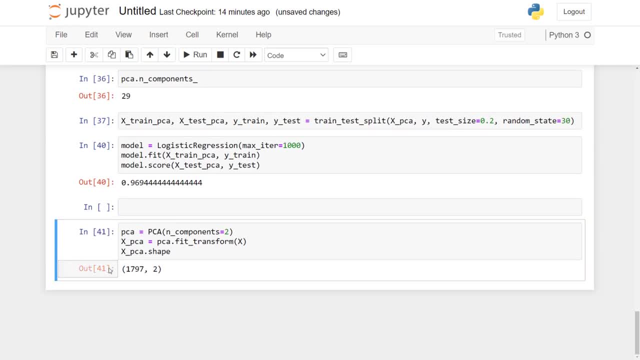 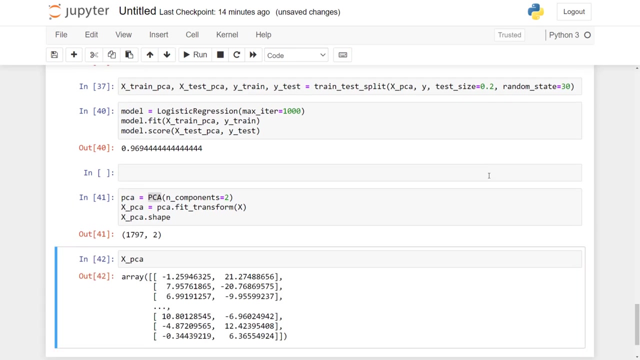 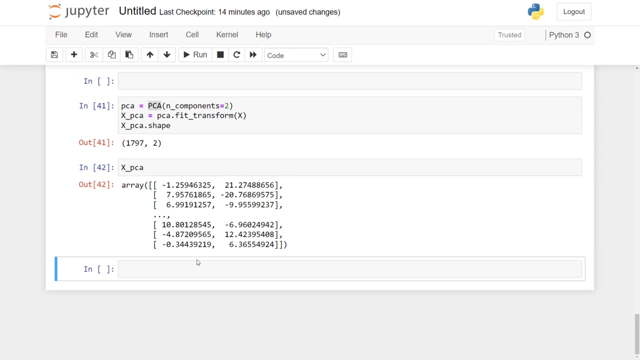 XPCA dot shape. now we are telling that we want two components. okay, so it. it will identify the two most important features. but here see, let me see, so see, every data point is just two features. now, did it capture enough information? we are not sure. when you print, explain variation, variance ratio, you are 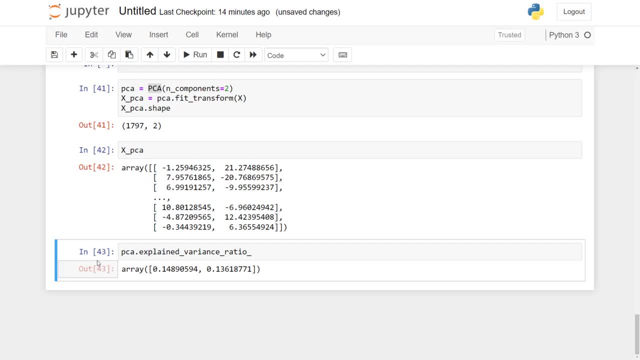 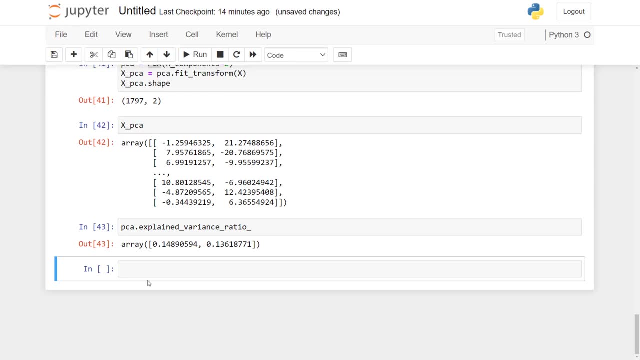 capturing 14 percent and 30 percent- around 27- 28 percent information. so naturally, when you use this data set to train your model, the accuracy is going to be low. so I'm just going to like same code, but I'm using the new PC and the 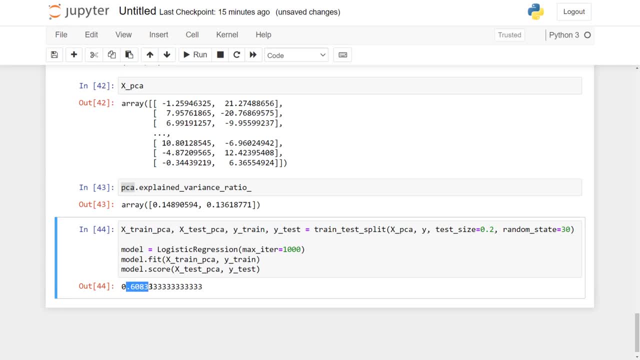 new data frame and when you train the model you see the accuracy is reduced to 60, 60, point 83. so you take a hit. but the benefit you got here is your features are only two, so your computer can be. computation can be very fast. so 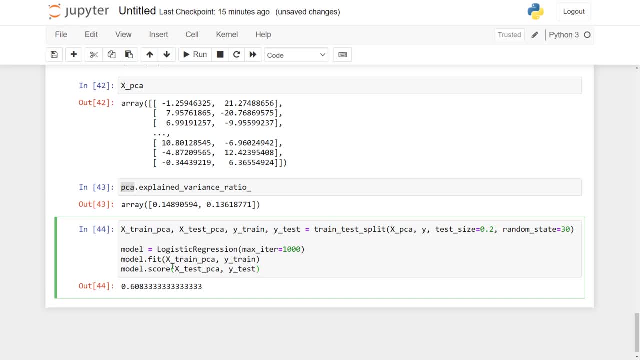 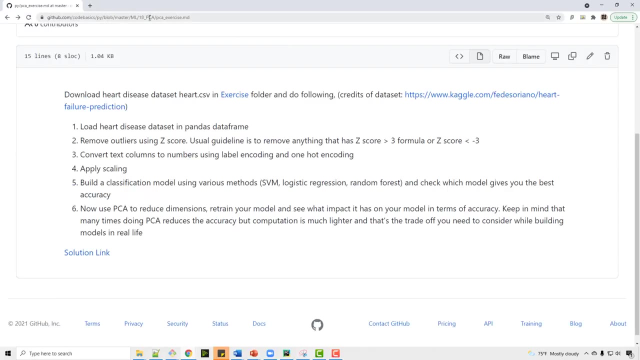 you can decide what accuracy do you want, and then you can reduce your dimensions accordingly. so that's all I had for this video. now let's move on to the most important part of this tutorial, which is an exercise. I'm going to provide a link of this exercise below, but it's very important, friends, that you work on. 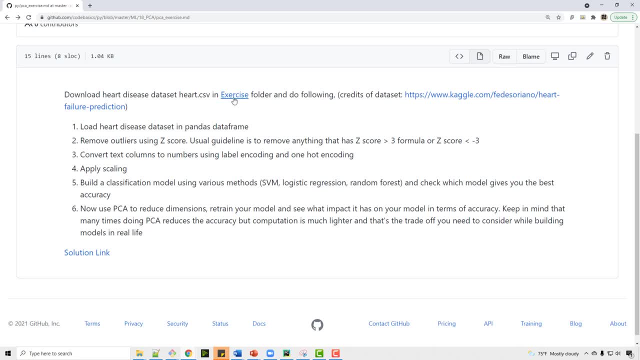 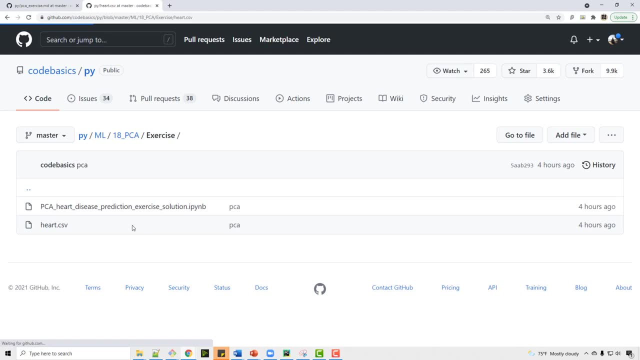 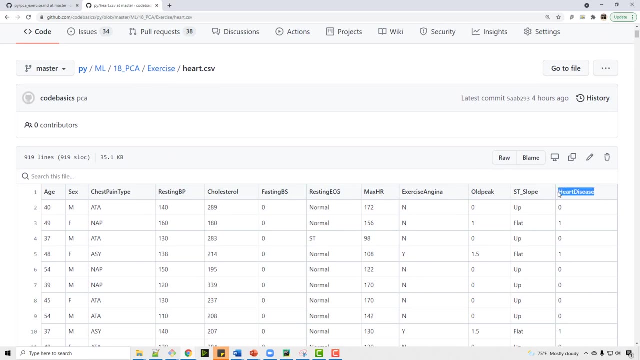 exercise and I have given a very good exercise. there is a data set which you can download from Kegel or you can see if you click on here. there is this heart CSV, and so there is a data set for heart disease and using this data set you need to predict if the person has heart. 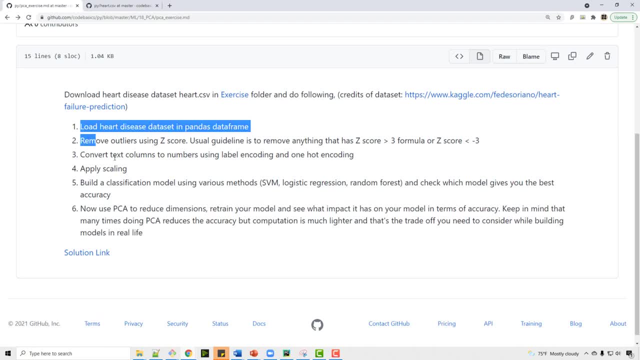 disease or not, and you are going to use PCA. so work on all these six aspects of the exercise and let me know how it goes in the comment. post below your solution, your github link, whatever- and if you like this video, please hit the like button. you have any question? post in a comment below and if you like this video, share it with your friends.